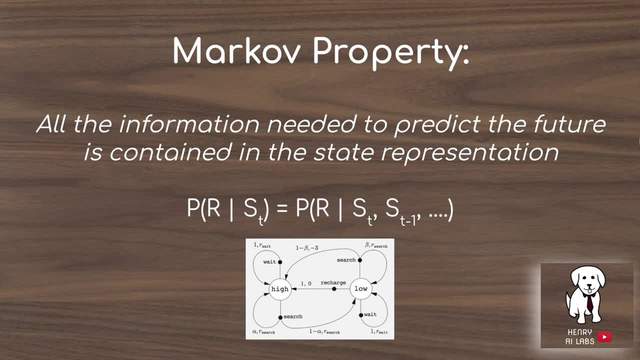 Markov decision process is the Markov property. So what the Markov property is is? it basically says the. all the information that you need to predict the future is contained in the current state representation. So using conditional probabilities shown here, we can summarize the Markov property. 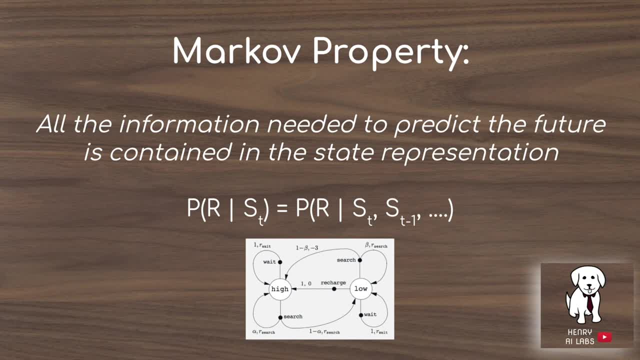 as saying that the probability of the reward given the state at this time step, say t, is equal to the probability of the reward given the current state, the previous state and then all the previous states that have ever existed in time. So basically, to just summarize it, the Markov property says that all the information you need is given in 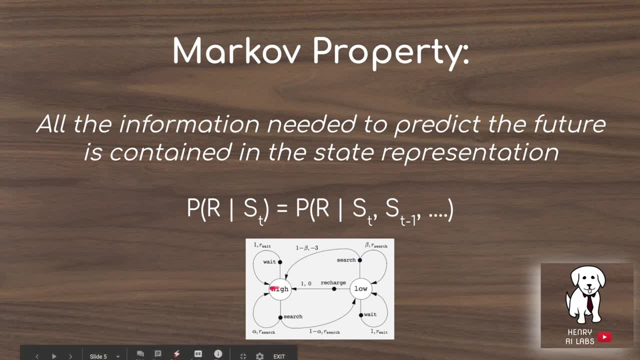 the current state. So in the example of our recycling robot, it doesn't matter when the robot is in the high battery charge state. it doesn't matter whether it just came from high or if it just came from low and has just recharged, or if it has just come from waiting. all that matters is the current. 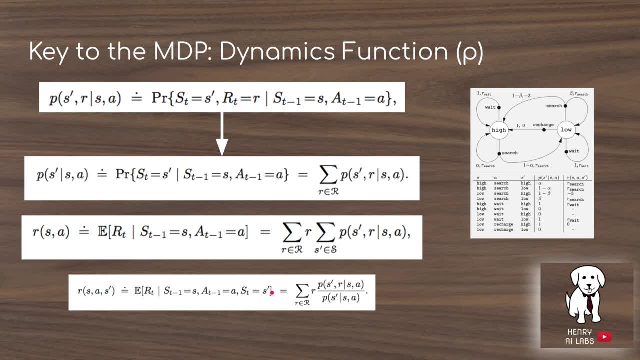 state to predict the future. Another key of Markov decision processes are this is this dynamics function p. So the dynamics function is basically telling you how the environment is transitioning with respect to the different actions you take, as well as the rewards you can expect to get as it's transitioning from state to 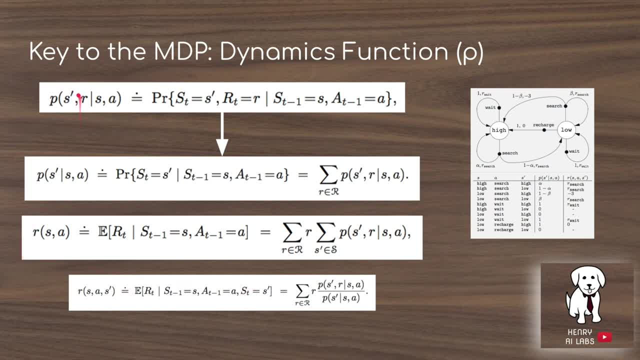 state with respect to the action taken. So from the for argument dynamics function, which is, give the next state and the reward given the current state and the action taken, you can also derive other things you might want to know about the Markov decision process, such as the next state. 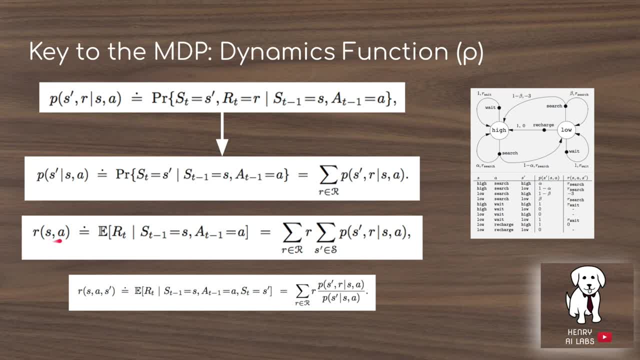 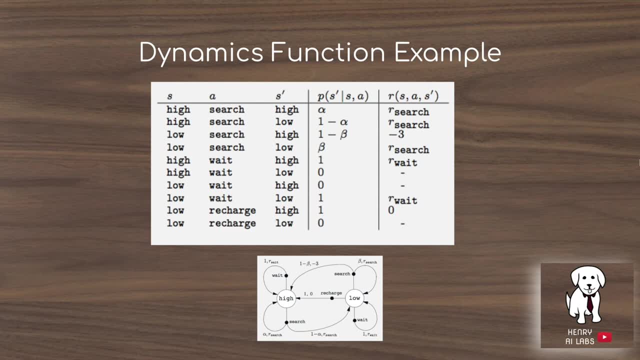 probability given the state action pair- the reward for a state and action and the reward for a state action next state to both. The dynamics function of a Markov decision process is probably better explained through the use of a concrete example like the recycling robot. So in this case we're looking 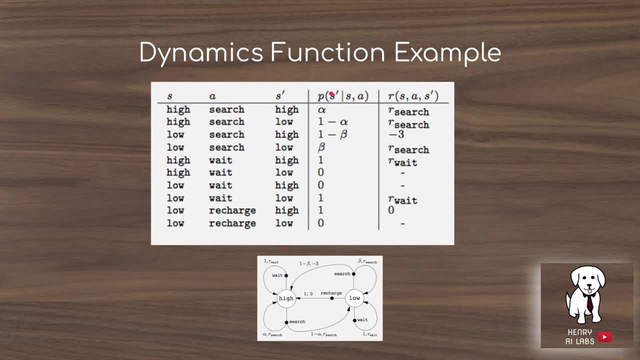 at a table of state action and next states and the probability of going into this next state given a state action pair and the reward achieved by this state action, next state tuple. So the first entry of being in the current state high and taking the action search. 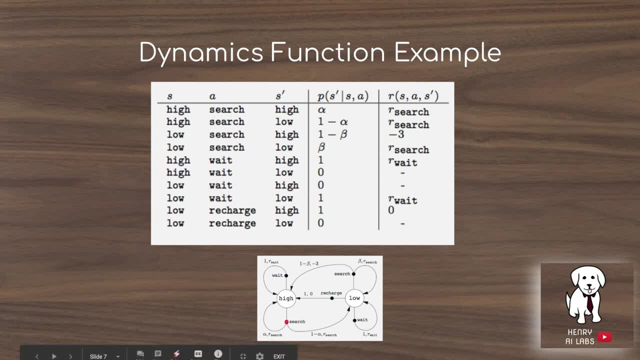 Corresponds to this path on the Markov decision process illustration. So we're in the current state of having a high battery charge and we just decided to go search for trash. So if we find the trash we receive this reward. our search in both cases. But we also have this probability of 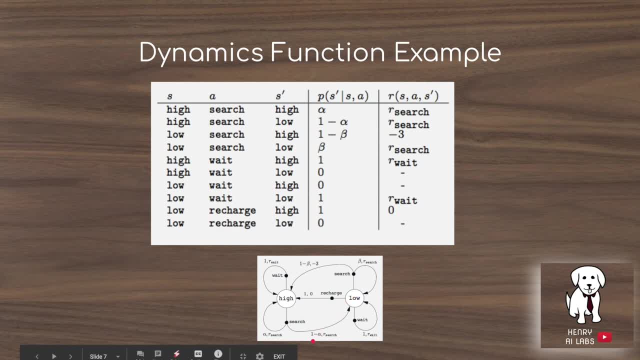 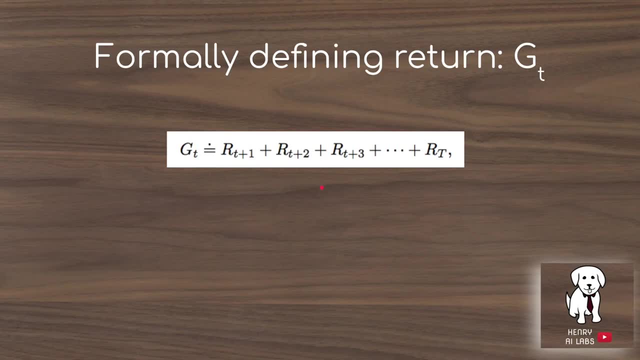 transitioning from the high battery charge to the low battery charge with this one minus alpha parameter, or essentially, staying in the next state of high with this alpha parameter. Now that we have an understanding of the transition probabilities of going from one state to the next, with respect to the actions we take in the state we're currently in, 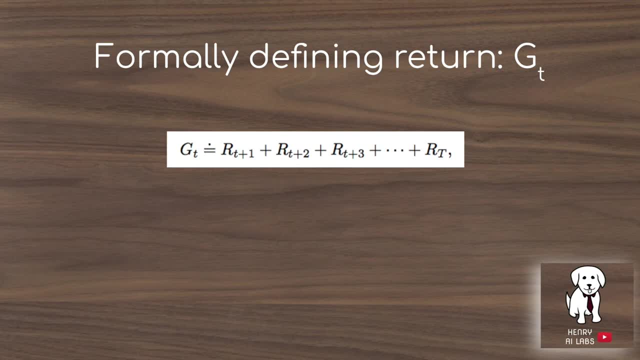 So we're going to formally define our idea of expected reward or return, denoted G sub T. So, as we've seen in many of the reinforcement learning cases, we constantly receive a reward from the environment at every time step. So the return of the 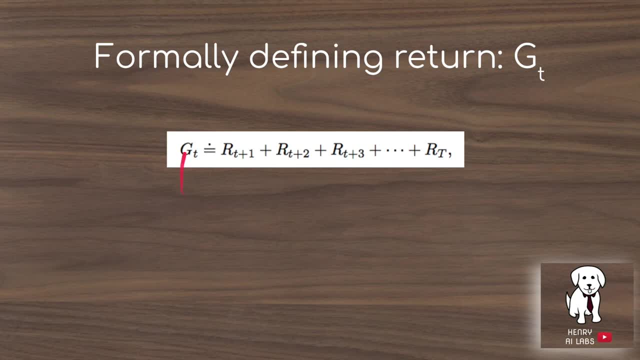 expected reward in total is the summation of these rewards we achieve at each time step. So in this case, if we have an episode with T time steps, it's just a summation of all the rewards up to time step T. So there are two different kinds of 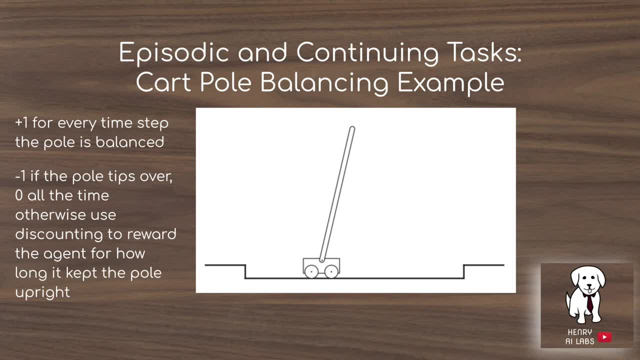 tasks that we're going to formally define and distinguish from each other, And that's episodic and continuing tasks. And we'll use the cart pull balancing example to show how you might structure cart pull balancing as an episodic task or a continuing task. So if you've 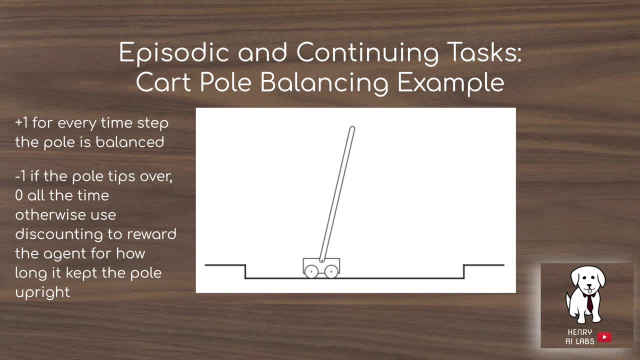 messed around with the open AI gym. this is an episodic implementation of the cart pull balancing problem. Basically, you get a plus one reward for every time step the pole is balanced And when the pole tips over, the episode is ended, and then it just. 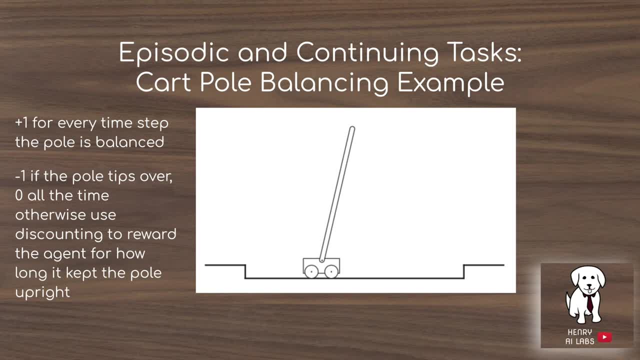 restarts back to the middle, And this is how the open AI gym allows you to interface with cart pull balancing. But another way of doing it might be to have a continuing task where the reward is zero all the time And then minus one when it tips over. So we'll use this idea of discounting in order to reward the agent for keeping the, the pole. 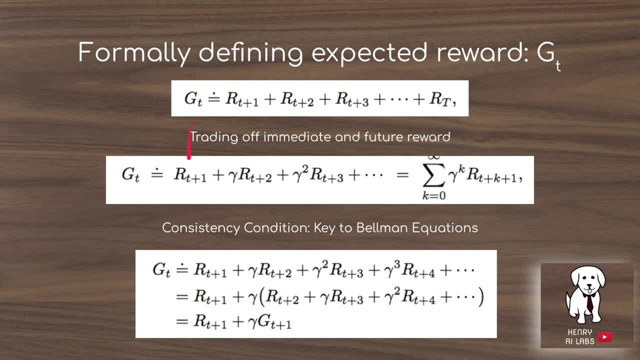 balanced for many time steps. So this is done with this gamma discount factor. So we've seen this idea of return g sub t as being the summation of rewards over a series of time steps. So now we're going to trade off immediate and future reward through the use of this. 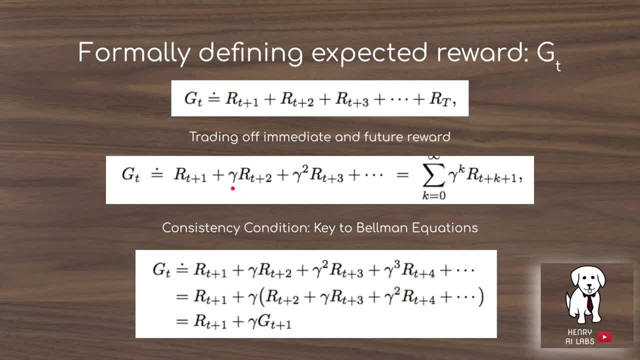 gamma parameter. So basically, if you imagine the gamma parameter is closer to one like 0.9, then is your 0.9 plus 1 equals to 10.. 0.9.. squared is 0.81, I think It's not so discounted. But say the gamma is 0.5, then gamma squared is: 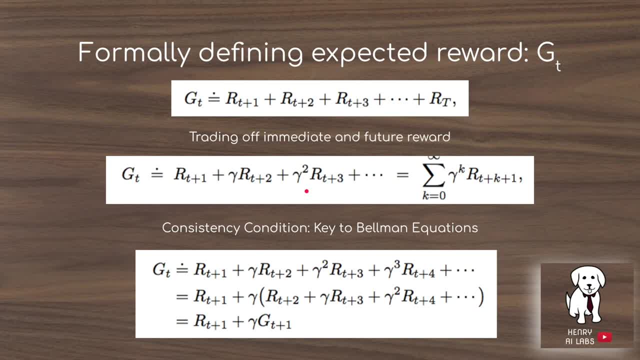 already 0.25.. So you see how gamma gets closer to zero. the future rewards matter less and less to the overall return of the agent. So, then, one key idea with this new notation of introducing discounting is that we can factor out the gamma from a sequence of rewards at different time steps. 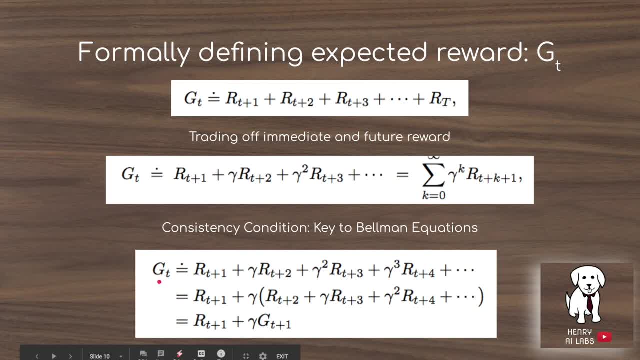 using this notation to have our return is equal to the reward at the next time step, plus the discount factor times the expected return at that next time step. And this consistency condition of g sub t equals r sub t plus one plus gamma times g sub t plus one is the key idea to the 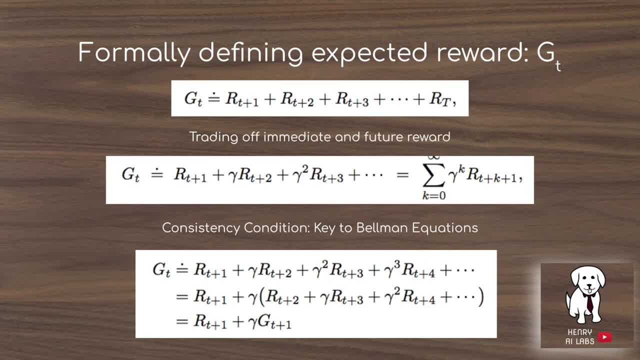 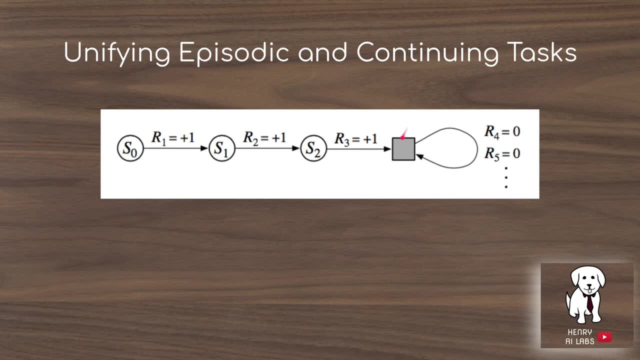 Bellman equations, which are one of the most important ideas in this chapter. In addition to discounting rewards, we can unify episodic and continuing tasks by using an absorbing state in our market. So what this gray box represents is converting an episodic task into a continuing task by just having 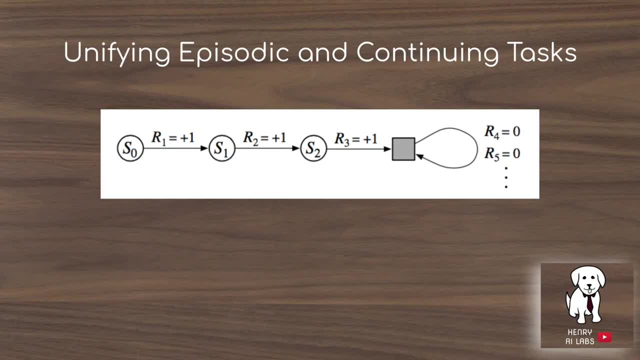 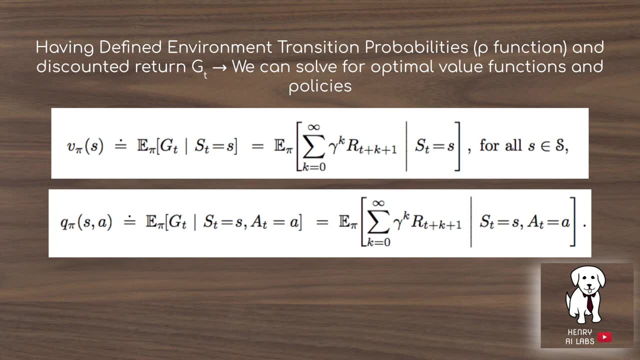 the end of the episode, loop infinitely and receive zero reward at every time step. So now that we have this idea of our discounted return and our transition probabilities, we can solve for the optimal value functions and policies using this idea of the Bellman optimality equations. So the Bellman 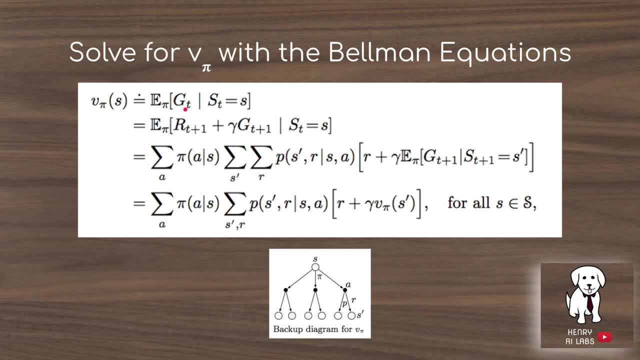 equations are basically this idea of breaking our current expected reward g sub t into the reward at the next time step, So we can solve for the optimal value functions and policies using this idea of breaking our current expected reward g sub t into the reward at the next time step, Plus the discount. 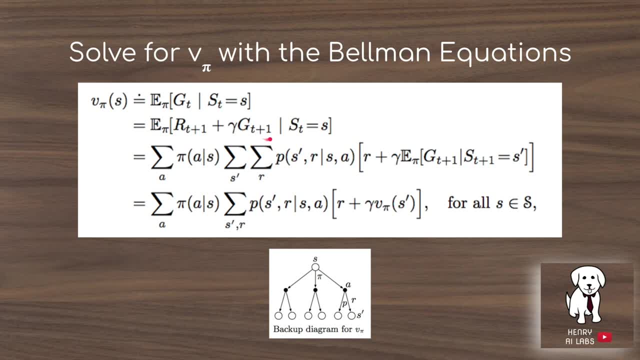 factor times the expected return from that state. So this is probably the key idea here to the Bellman equations is basically, you're computing the expected value of this state as a function of all the next states that it can transition into. So it's an idea derived from dynamic programming of you. 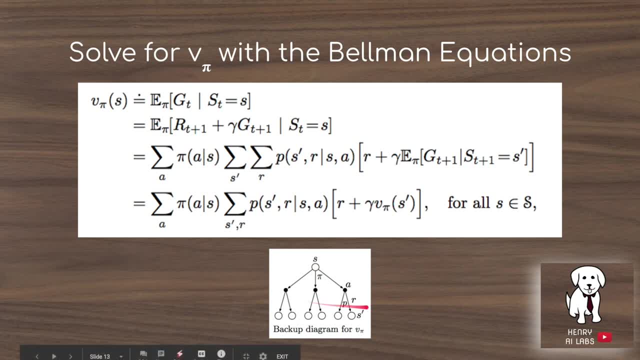 know shortcutting the equations needed by just using this one step look ahead. So that's why we see things like the backup diagram for the value function of this policy. pi at state s is just given on the next states it might achieve with respect to the different actions it can. 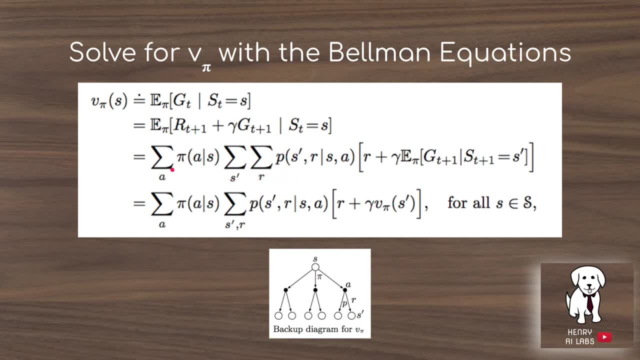 take. So all these details of the equation show is just the policy, meaning the action it takes, given the state, and the summation of the next states, basically the probability distribution over the next states, and rewards given this state action pair. and then we have our reward at that step plus the 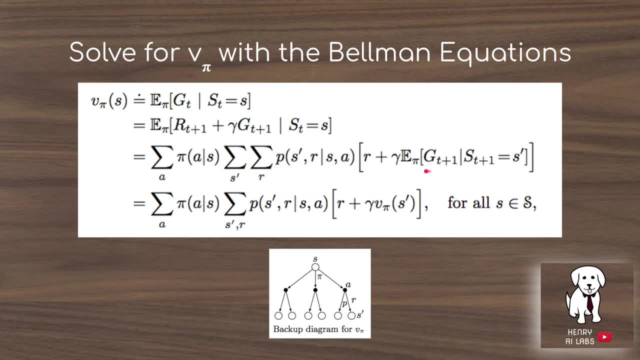 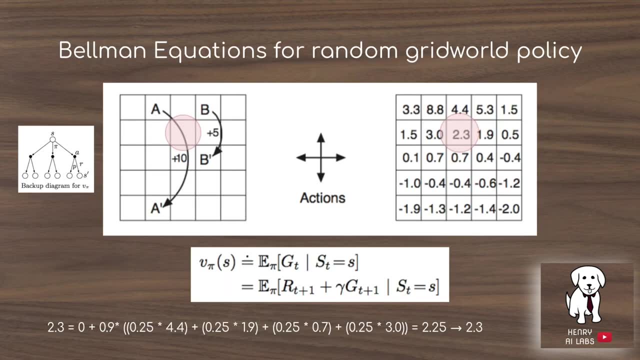 discount factor times the expectation of our future rewards from this new state S prime. Now we'll look at a concrete example to show how the Bellman equations can be used to find the value of every state given a certain policy. So in this case, our policy, or our mapping from states to actions, is random meaning. 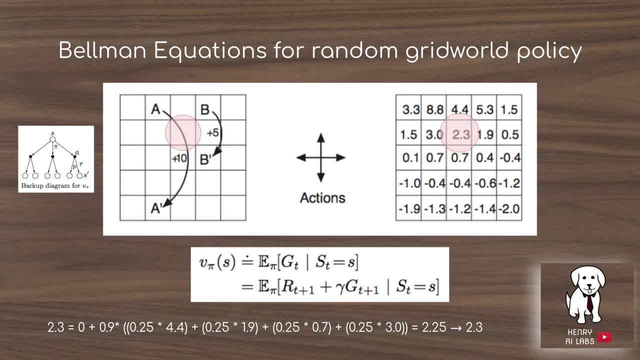 that we're choosing up, right, down, left, all with the same probability of 0.25 shown here in the calculation. So what the Bellman equation will do is we'll solve for the expected return of a state. in this case, we're going to look at how. 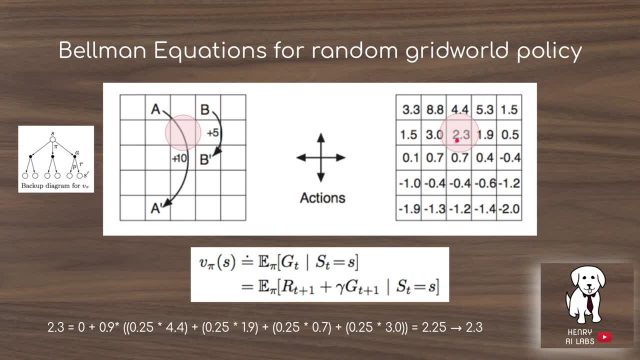 it derives 2.3 for this state as a function of the reward for that state, plus the discount factor times the expected return of all these subsequent states that it might achieve. So we're going to look at the number of states that it might go to and then the probabilities of it going to. 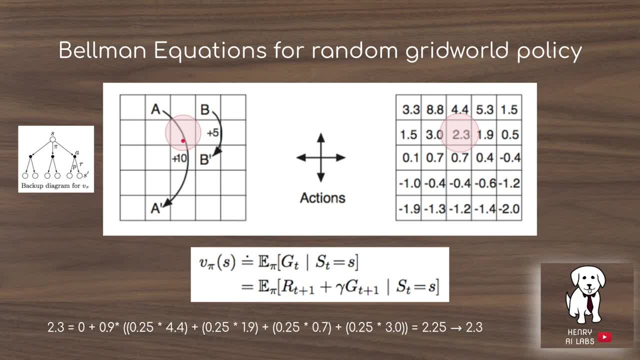 that state. So when we're in this middle state, we receive zero reward. we only receive reward when we're on A transitioning into A prime or B transitioning into B prime, or if we fall off of the map, we receive a negative reward. So from here we look ahead to our subsequent states. we can either go here: 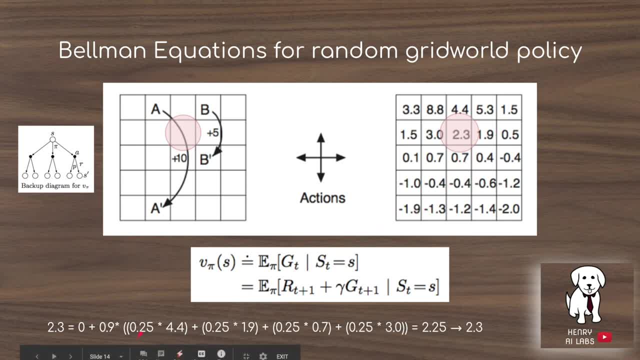 here, here or here, So from these different states, all with the same probability of 0.25. of transitioning into this probability, we have this summation, which is our sub t plus 1, and then we multiply it by a 0.9 gamma discount factor, and then we 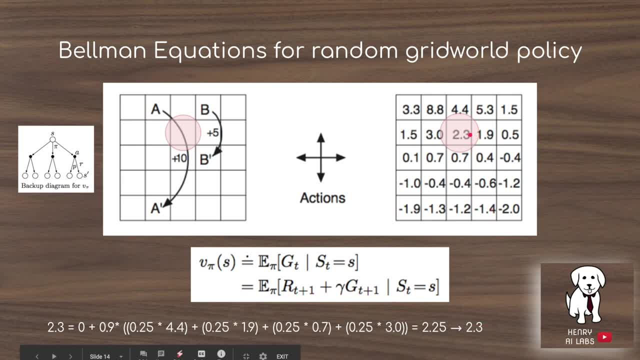 add it to the reward at this state and this gives us our estimate of 2.3 of for this state or the value of this state, using the Bellman equations, looking ahead one step to these subsequent states and using those to evaluate the state at the current step In the grid world example, we're looking at the 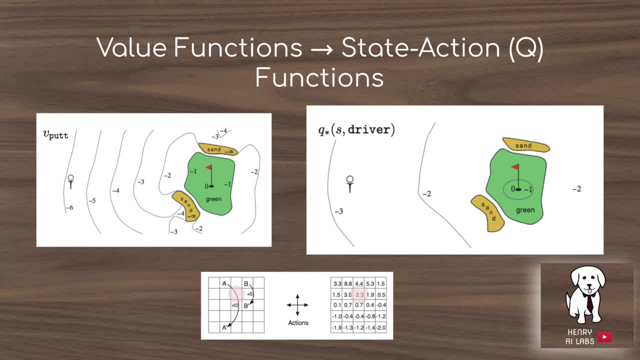 estimating the values of each state and then with respect to these different actions of moving up, right down or left. but it's also helpful to have an understanding of difference between value functions and then state action functions. so in the example of the golf problem, we have the value function, if all. 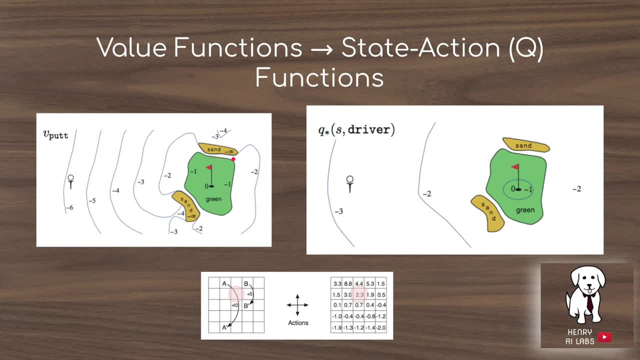 do actually take is to putt. we have this kind of contour map of our expected rewards at each location of the map. compared to if we have this action of using the driver, we see a different kind of contour map where, in this case, it's better to use the putter, but we're still using the driver compared to the putter. so this golf example is really a situation where you have one of the same sides, different sides want to use this Achaca driver to achieve the value against the putter. so the maneuver here is a line advantage. here when we use a linear, slight interaction, the agg powerful advantage of this balance which makes 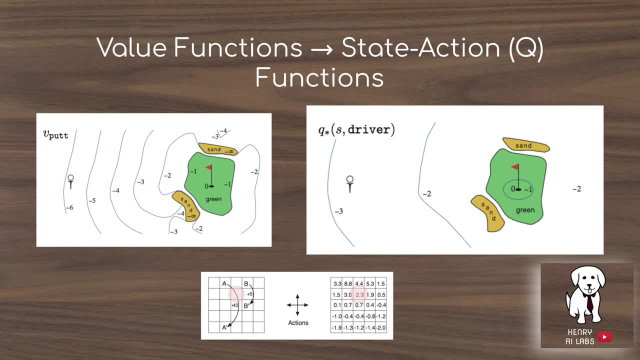 we not only have to most of the occasions here, but you know we could probably use it further over time to calculate the difference, to move the value. just good to get a concrete example of the difference between value functions and then how adding different actions can change this with the state action. 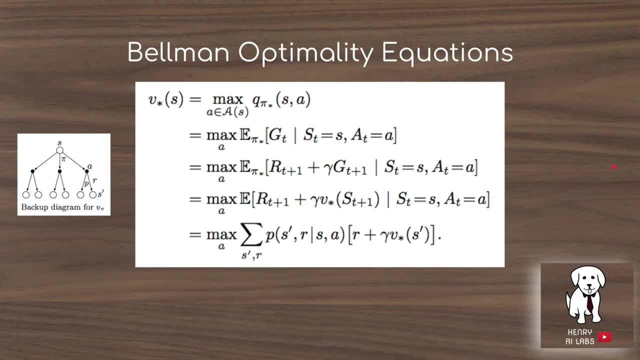 functions or the Q functions. So we've seen how the Bellman equation can be used to compute the values of states as a function of the successor states. but now we're going to look at the Bellman optimality equation, which is a way of solving for the optimal values of the, of the states in the, in the environment and 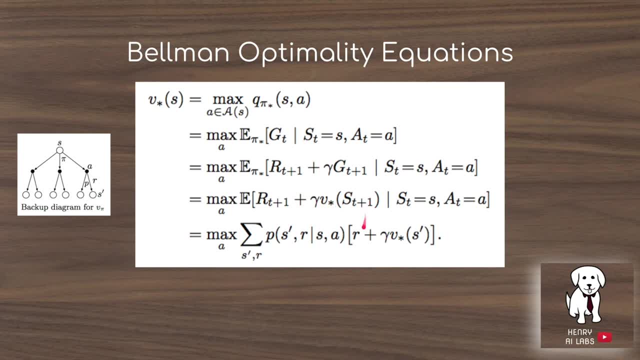 this is denoted V sub star, as the t plus one, or V sub star of s. So basically, what this is is taking the max a, or meaning taking the action which is the, you know, has the best reward at each of the states, in order to maximize our reward. 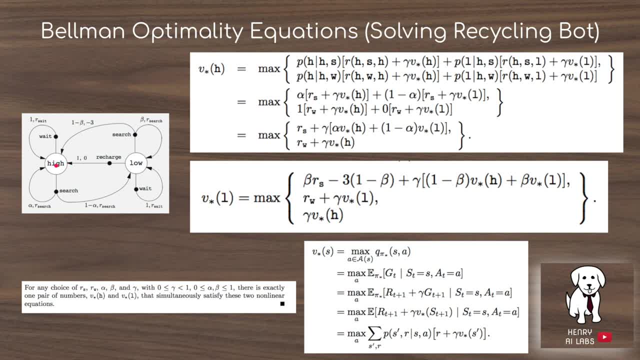 So, from the state where we have a high battery charge, we either take the actions of waiting or searching, and that's given right here in the V star of H or the optimal value function estimate of H as the maximum reward with the actions that it can take. So the way this top. 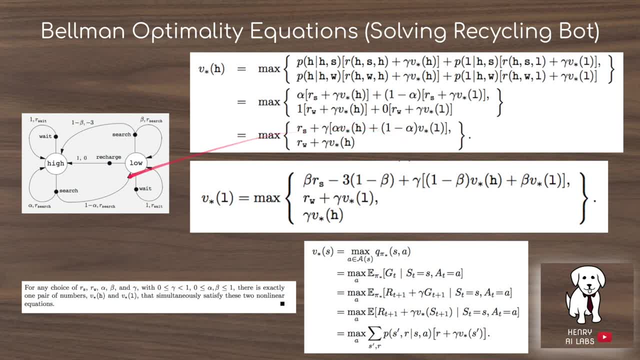 line of the argument is defined is: this is the reward given by searching, plus the gamma times the for the discount factor, times the expected reward for where the next state might be. So, for example, we have the alpha probability of returning back to this high state. so then we're back in the same H state and we have our 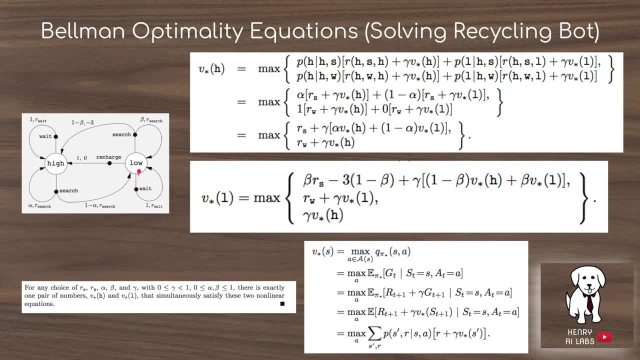 value estimate of that state. but then we also have the 1 minus alpha probability of going into this low battery charge state. so we have our value estimate of that state And then, contrarily, we have the weight decision or the action where we receive this reward, R sub weight, and then we have, plus the gamma times the expected 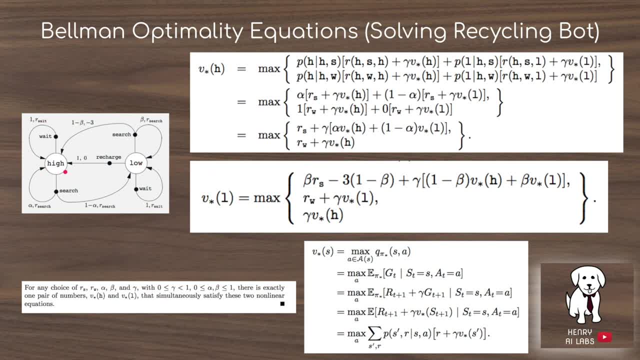 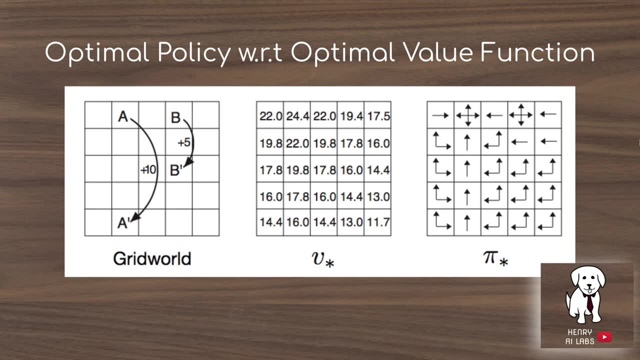 return for the new state that we're in, which, in this case, is always going to be returning us to the state of high battery. Using the Bellman optimality equations leaves us with this system of equations that we can use to solve for the optimal values at each state. 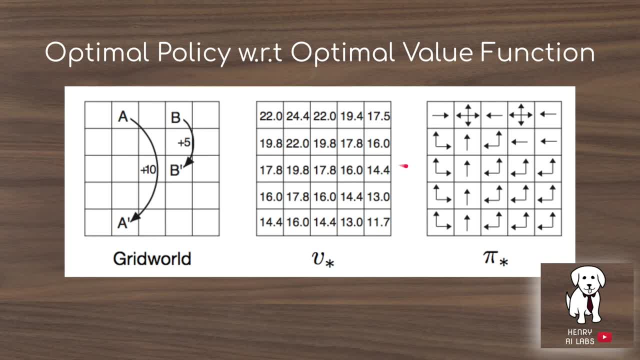 So once we have this table of the optimal values at each state, it's easy to construct a policy, an optimal policy, which is basically just taking the greedy decision to move into the state with the highest value. So, for example, if you're in this state of 19.8 of the value estimate, you would move. 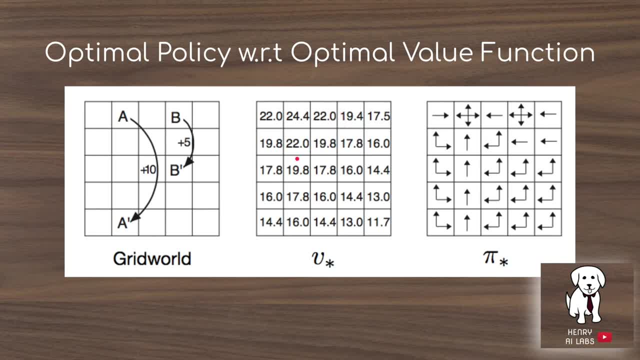 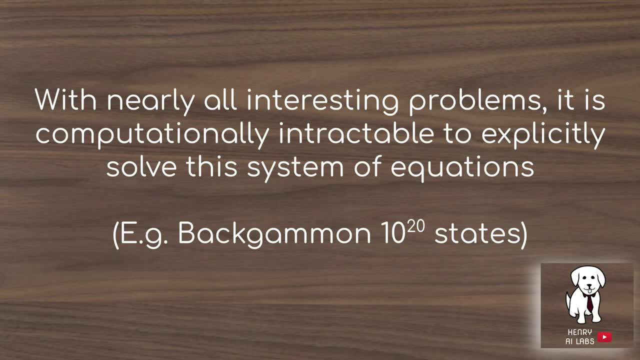 either up or left to the higher value state at 22.0.. So with nearly all interesting problems, it's actually computationally intractable to explicitly solve the system of equations like this. So in our recycling robot case we only have two states, so we can and only get three actions in the low battery state.